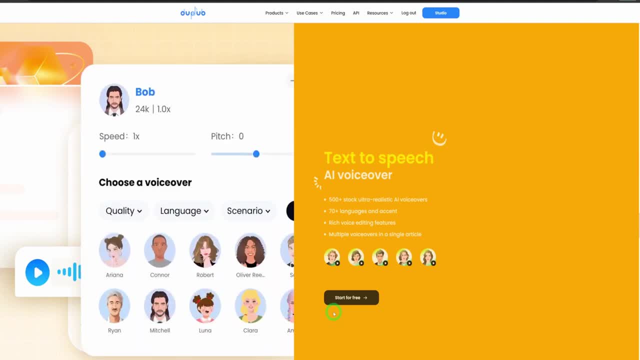 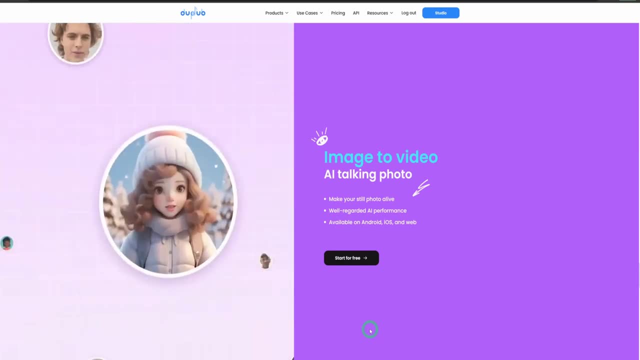 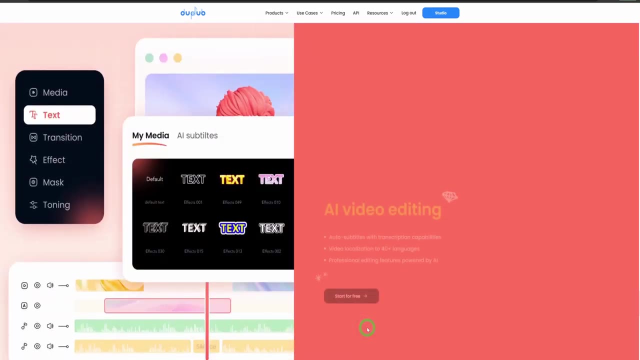 using multiple plethora of different voices, And it can be done in over 70 languages as well. And then it has the capacity to generate very intriguing AI arbiters through your images, like we have on this channel. And finally, it could do some amazing editing as well, Coming into their products. you could just do all tools. 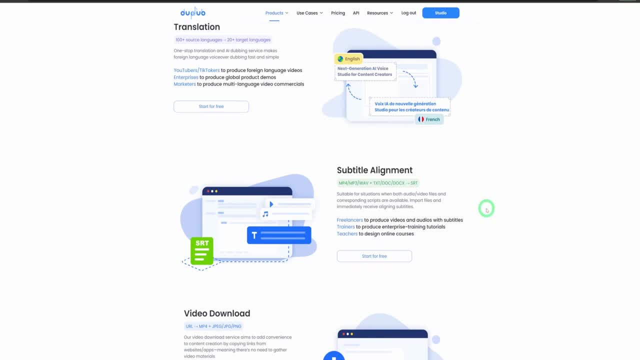 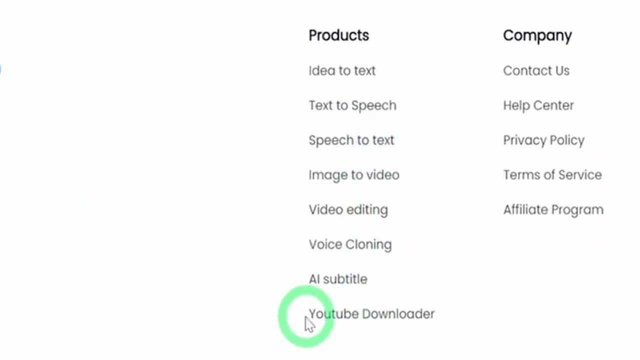 and it's going to give you a breakdown of all the tools they have And you could just sign in with your account, your email address- It is free- And then we'll go ahead at the bottom here where you have product, and we're going to click on text to speech And it's going to open up to this page. 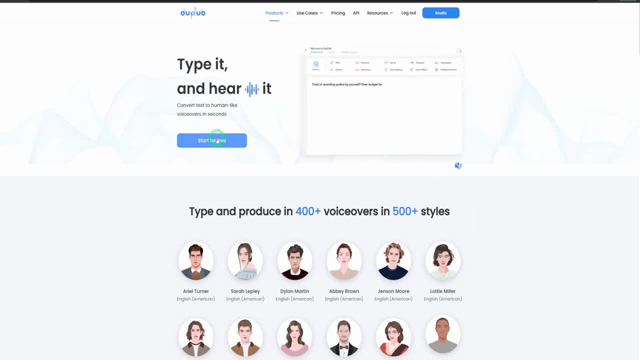 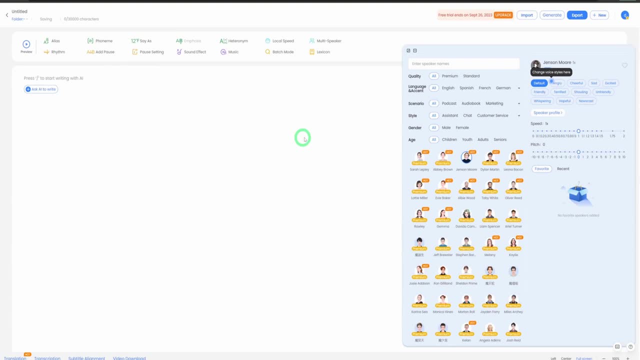 There's over 400 voiceovers and over 500 styles. We'll just say: start for free. I've already signed into my account. It's just going to log me into this page. What it's going to do is the right here. 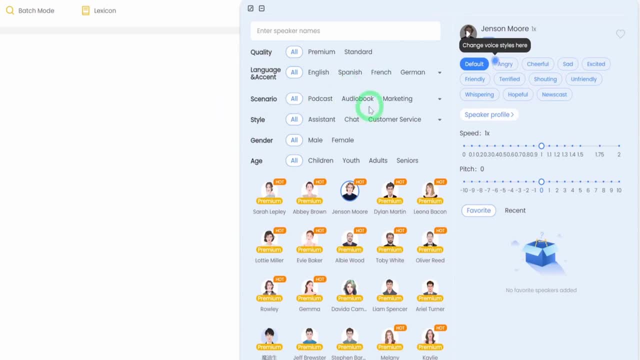 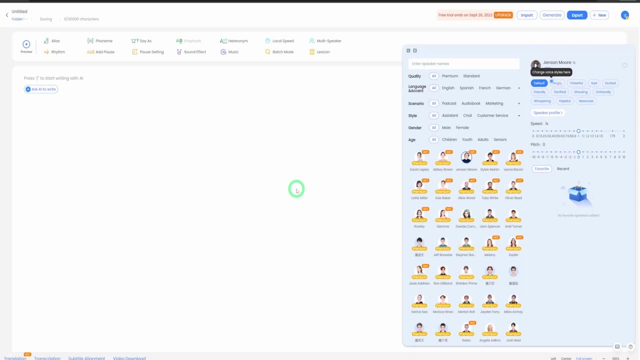 you would see different characters, the quality, the language, the scenario, the style, the gender and the age. You could use this to filter down the voice you want to use. And one good thing I like about the platform is that it has different features in terms of putting some aliases. 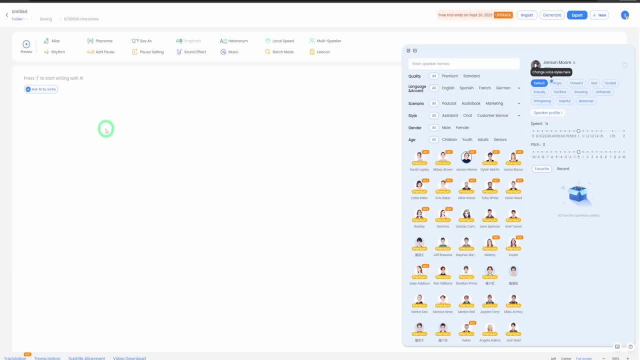 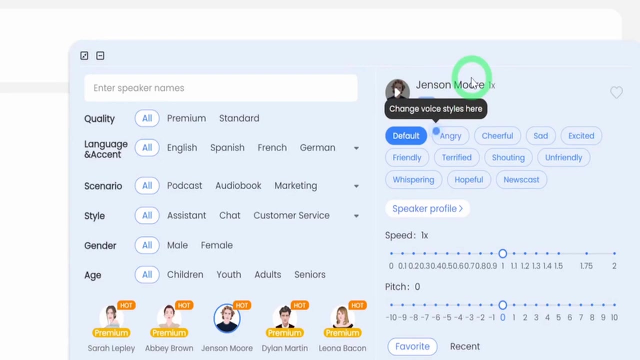 punctuations And, if you want, you could generate your script within DubDub and then generate the voiceover. But we've already generated our script. We'll just paste our script here And the voice I'll be using would be Jessin Moore. This voice is very cool for what we want to use it for. 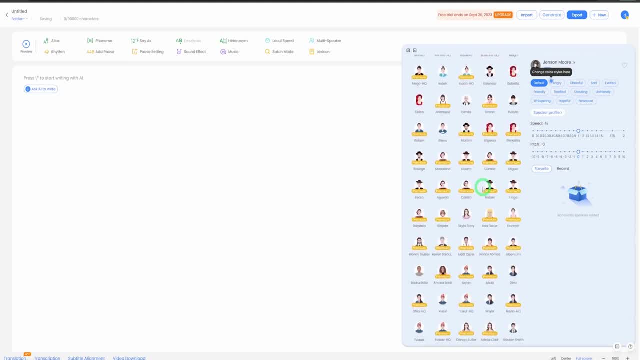 but you could play around to try out different voices they have. They have a lot of voices here. What we'll do is to copy and paste our first script and generate the voice, And that's the process we're going to take, And then we're going to go ahead and create our script. 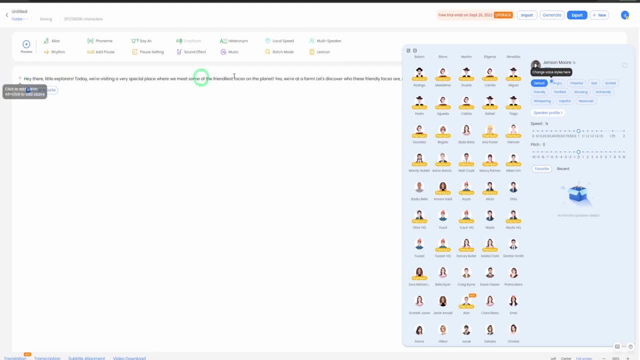 We're going to generate all the voiceovers for all the scenes. Just paste in an intro here and we'll go ahead to play this so you could see how it sounds. Hey there, little explorers. Today we're visiting a very special place where we meet some of the 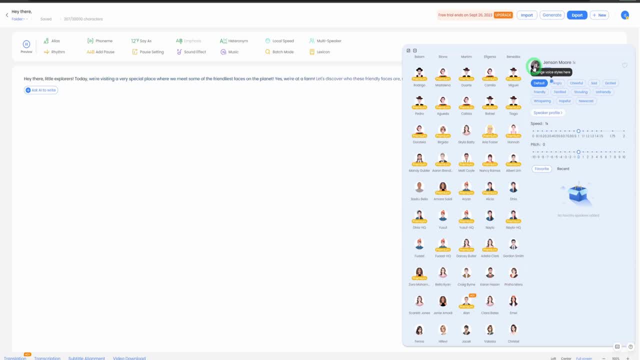 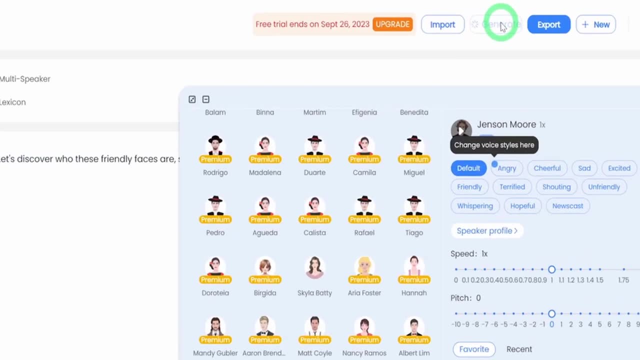 friendliest faces on the planet. Yes, we're at a farm. Let's discover who these friendly faces are, shall we? Okay, this is good. The next thing you need to do is just to click at the top here that says generate, and it's going to generate that voiceover. You just click on that and it's going to generate. 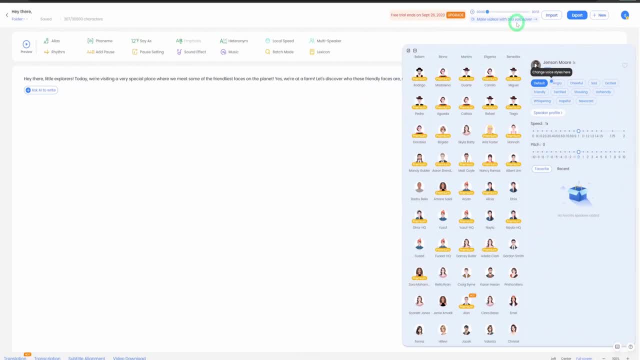 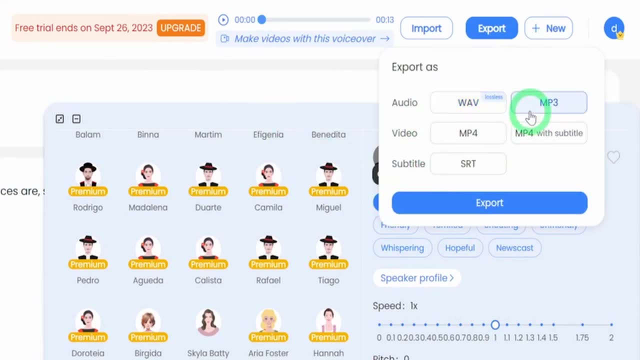 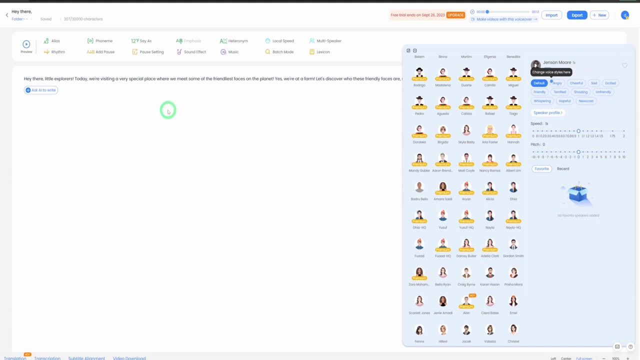 speech and it's going to generate that for you. And once it's done generating, just click on export and it's going to give you different options: wave, mp3, and so on. We'll just choose mp3 and click on export and that will be exported. You will do this individually for each scene. 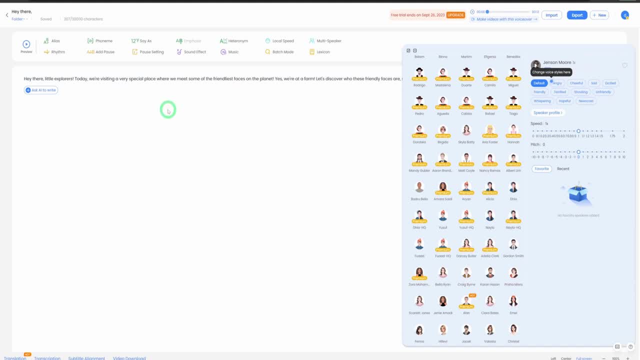 because we don't want to create a single voiceover, because we want to use it for what we want to do in the next couple of steps. To use DubDub, you could use the link in the description box. It gives you three days free trial and after that you will be able to create a single voiceover. 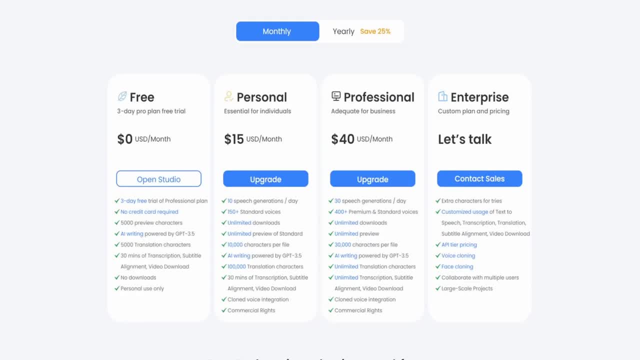 You would have to pay subsequently for the tool. To give you an idea of the pricing, this is the three days free trial. you could try Then for your personal plan. it charges you about $15 per month to use the whole platform and then so on. If you use the yearly plan, then it reduces. 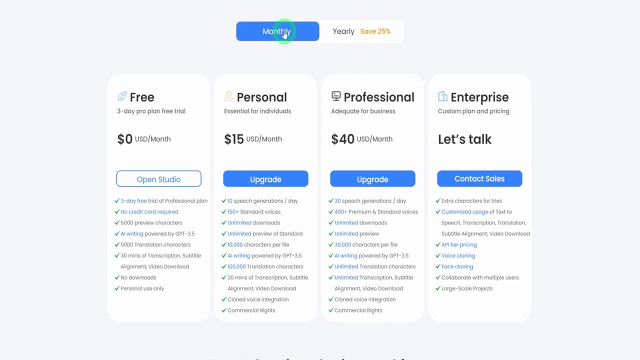 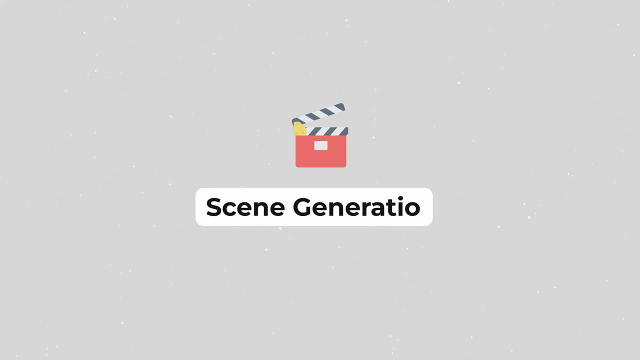 the amount that it charges you. Thank you, DubDubs, for sponsoring this part of the video. After you have done generating all the voiceovers for all the scenes, the next thing would be for us to create these scenes, And to do that, you'll be using Canva. Canva is free. You can create. 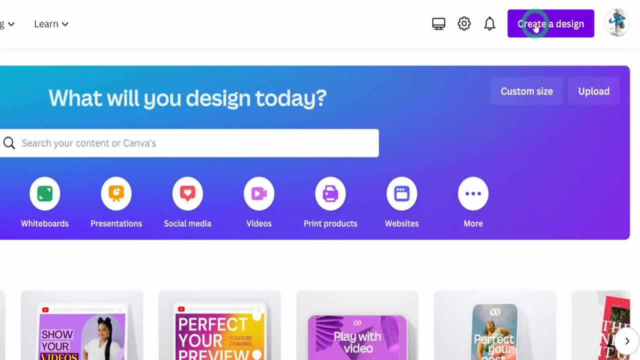 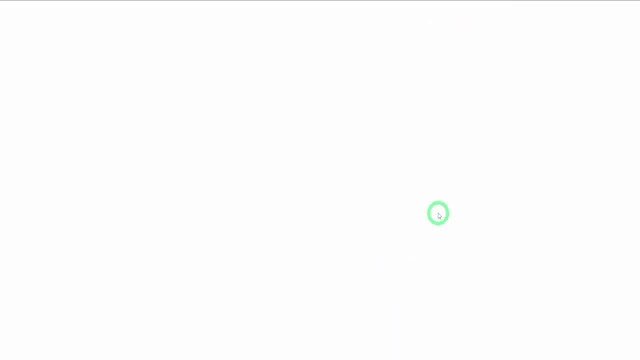 it for free, of course- Then what you could do is to click on after you have signed it into your Canva account, click on create designs and then click on custom size. We'll be using 16 by 9 inches because we want the same dimension as a YouTube video, And then we'll be putting the different 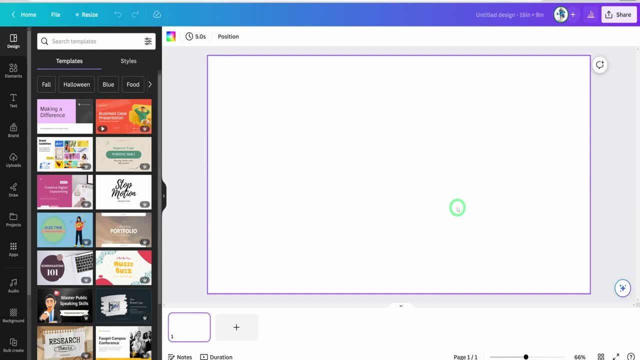 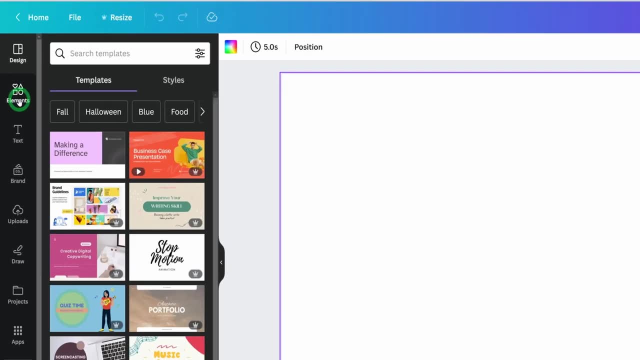 scenes. here For the scenes, what we'll be doing is based upon the story or the script that ChatGPT has generated for us. the first scene would be an opening scene of where a farm is. You just come into elements and search for. 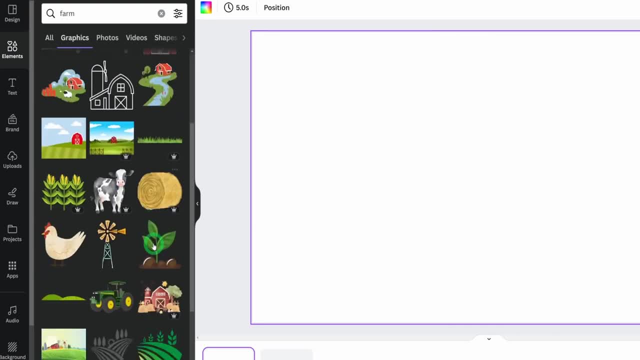 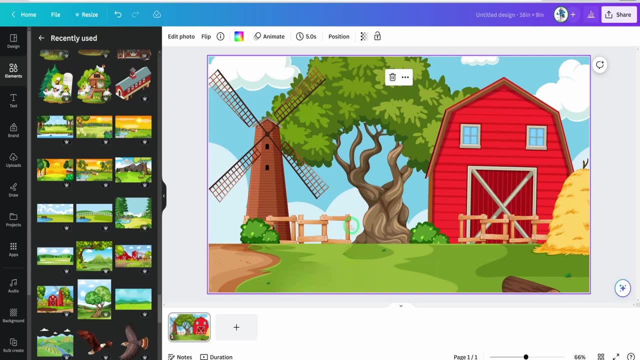 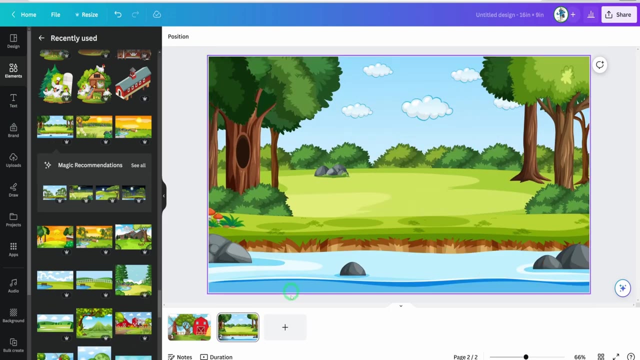 a farm and then try to use graphics to find the one that is very interesting to you. I found this one. This would be our beginning scene, For the next scene would be for where the cows are. We'll just use this. What we just do is set as background, And the third thing is where the chickens are. 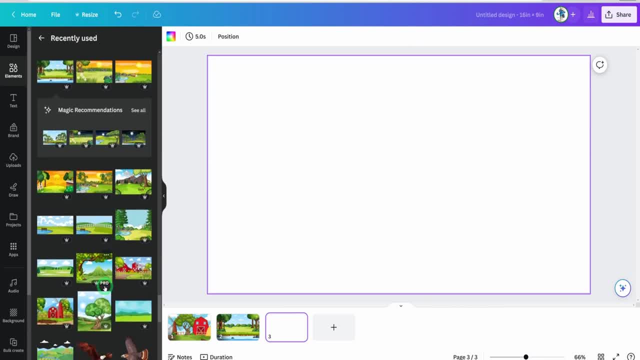 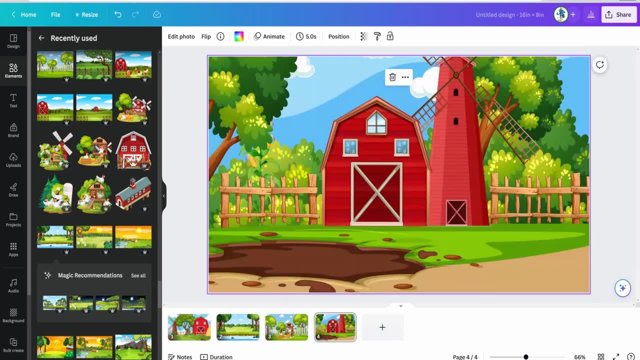 based on the script. We'll just use one that I have found already. Okay, The scenes are coming together. This is how you will go ahead to create all your scenes. Once your scenes are all set, like we have for scenes here, the next thing to 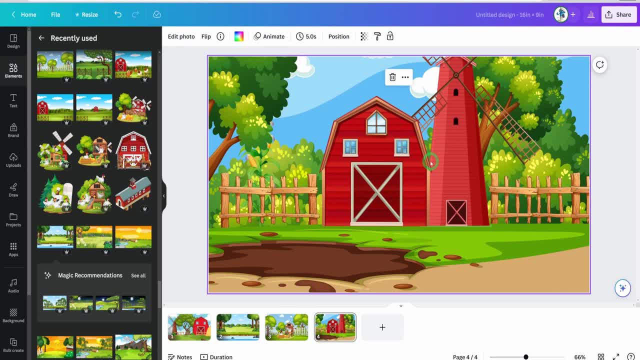 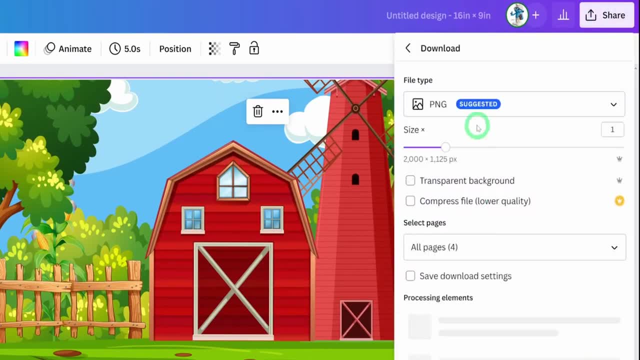 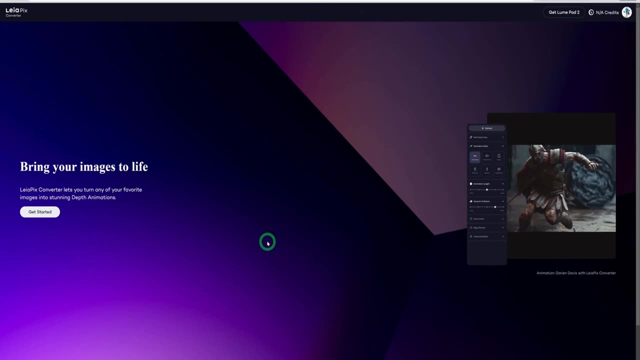 do is to download all these scenes as a PNG file and we'll be animating these scenes. before we add some couple of elements within the scenes, Just go to share and download as PNG and download all of them To animate the scenes that we just downloaded. we'll just come to layer pics Layer. 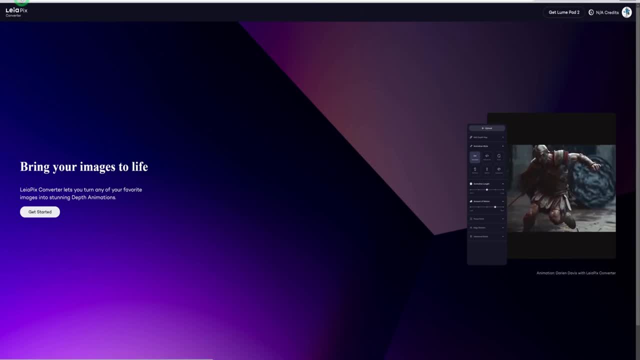 pics is currently free. From what I noticed- because I've talked about this tool on this channel before- is that you can choose between PNG and PNG2.. So having a PNG2, you can choose. from what i noticed, they started charging for it. they give you about 500 credits and after you have 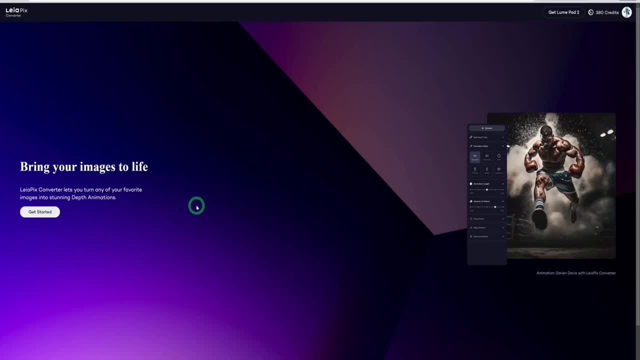 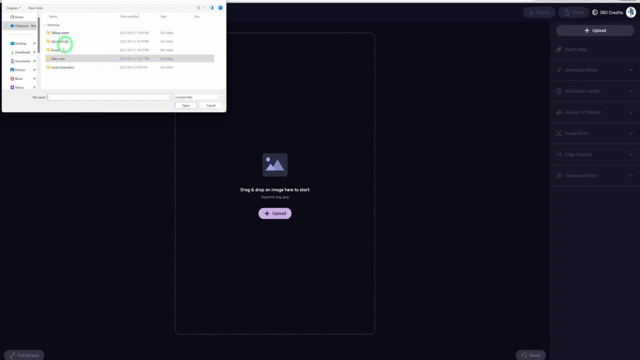 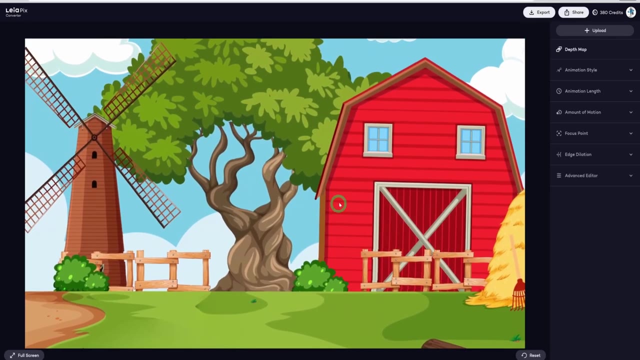 exhausted it, then you might need to pay for it, but now the 500 credit is enough to generate what you're looking for. you just click on get started and we'll click on upload. then we'll go ahead and choose the file that we want to put some movement to. so, as you can see, this has generated a movement. 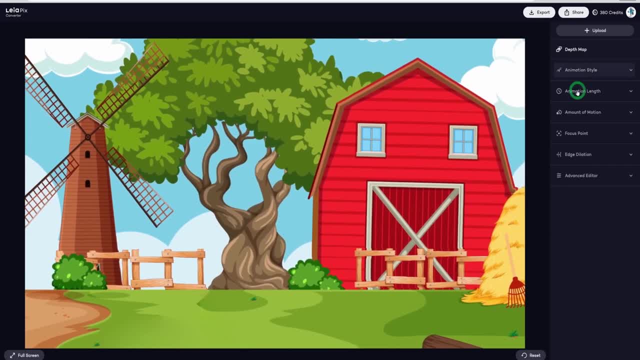 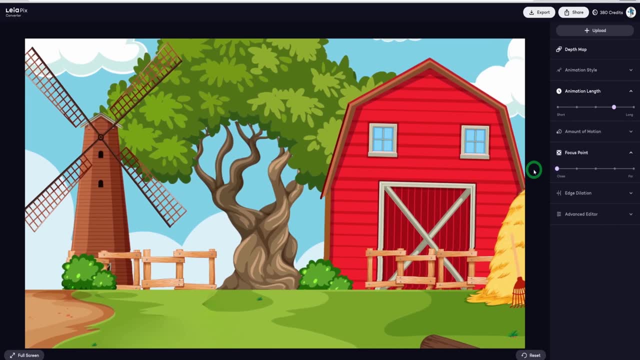 you could just change the style to what you want. just leave this style and the length. i will make it longer. and for the motion, i like how it is. for the focus point, i will just take it all the way down. as you can see, i like how this looks. the next thing is to click on export and it's going to 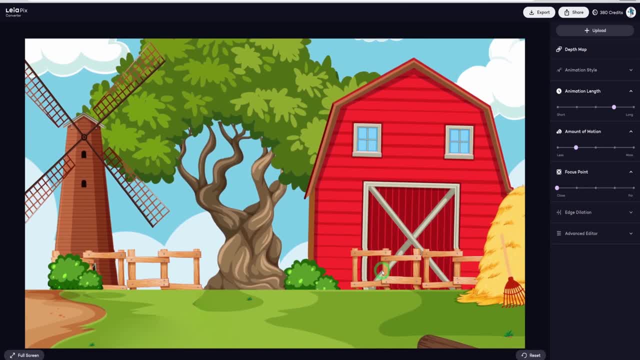 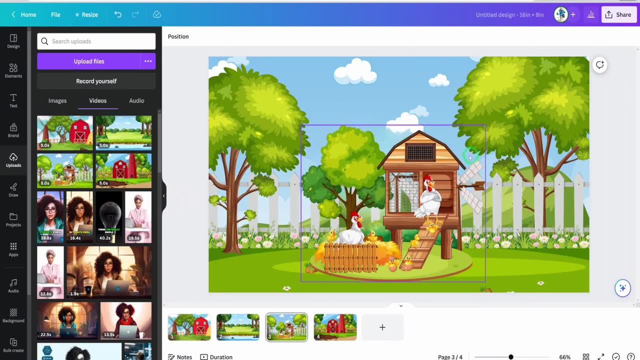 export this to my computer. you go ahead to animate all your scenes and save them to your computer. once it's done downloading, the next step is that we'll be uploading it back into canva and to open it up. we're going to go ahead and click on export and we're going to go ahead and click on. 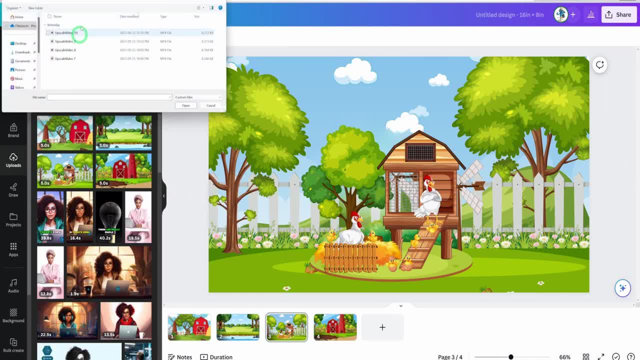 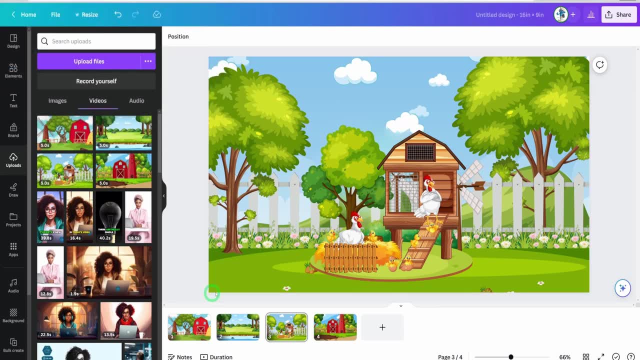 upload, that you just click on upload files and then select the clips that you have downloaded and upload them. i've uploaded these clips- as you can see four of them here- and what i will do is we're going to replace them with the static images we have. i'll just go ahead and delete this and 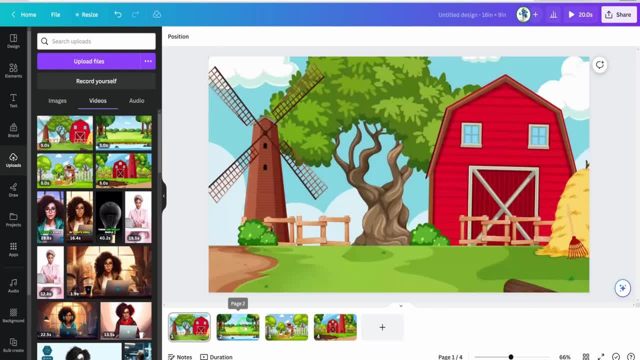 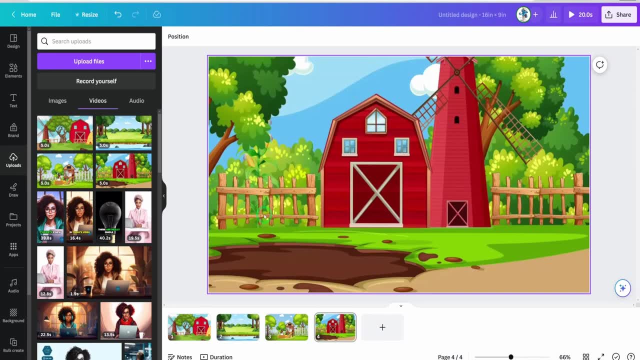 replace it with the moving one that we have and set background. you do this for all the scenes. this is moving set background. okay, now we have our videos all placed, i want to add some bit of moving elements within the scenes just to give it a bit of life. i'll just go to my elements as well and i'll be looking for 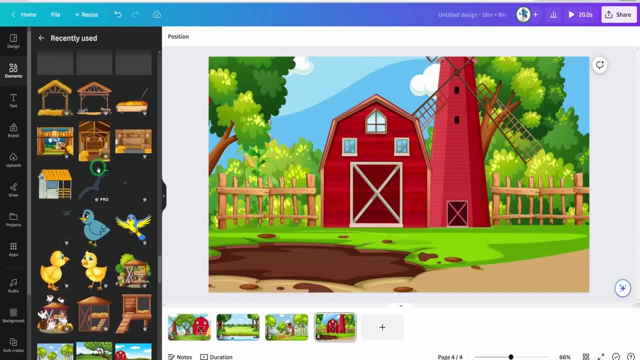 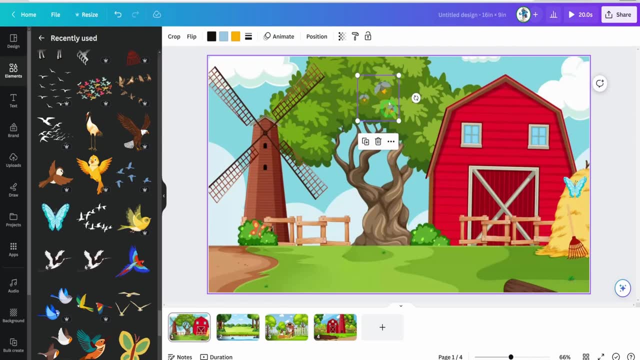 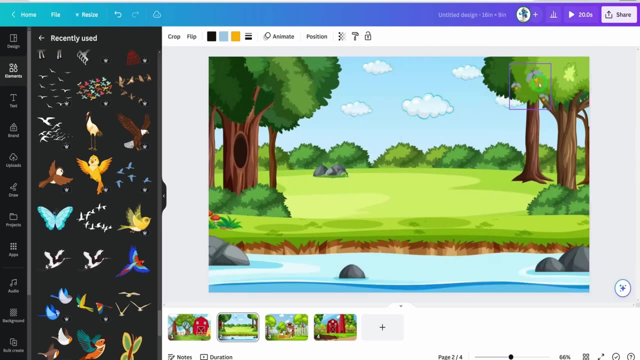 like butterflies and stuff, just to make it alive. i've gone ahead to find some butterflies that i placed here and, as you could see, i placed some other flying insects here and some butterflies as well. i'll repeat that in some scenes that i wanted to have something going. i'll just put it. 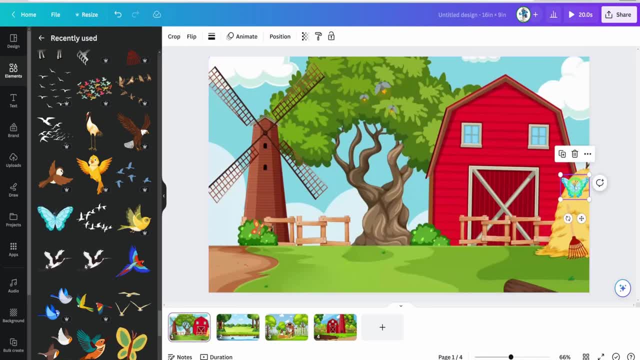 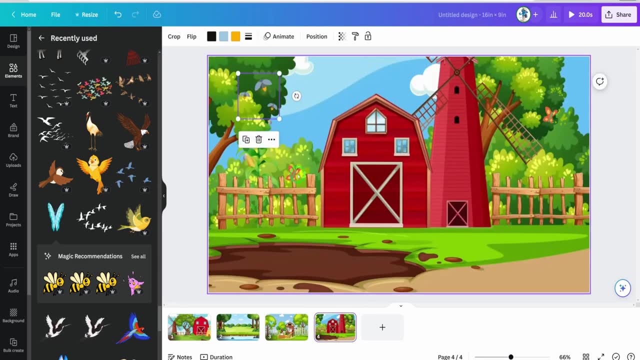 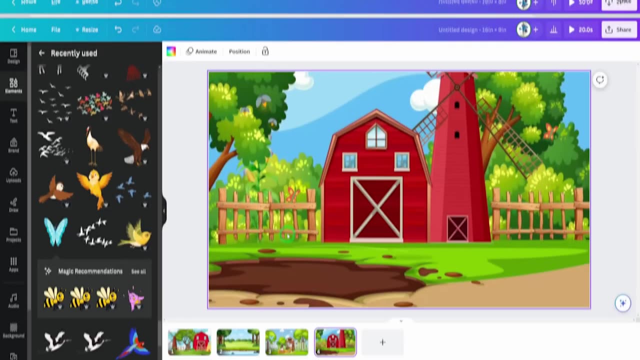 here. then for this, i'll just add some butterflies like i have here. i'll just put it here: we're good more somewhere. and then for this, i've added this as well: now that our scenes are ready, we have four scenes here. the next thing we need to do is to bring in all the voiceover that we have. 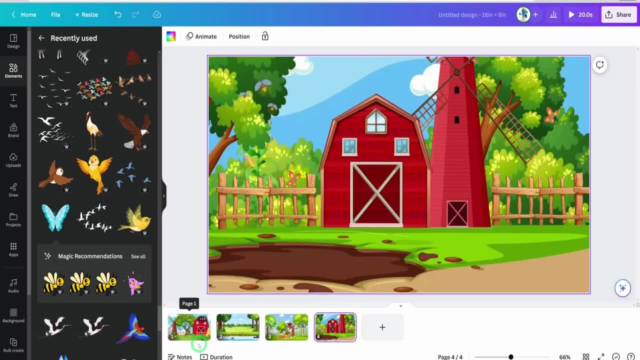 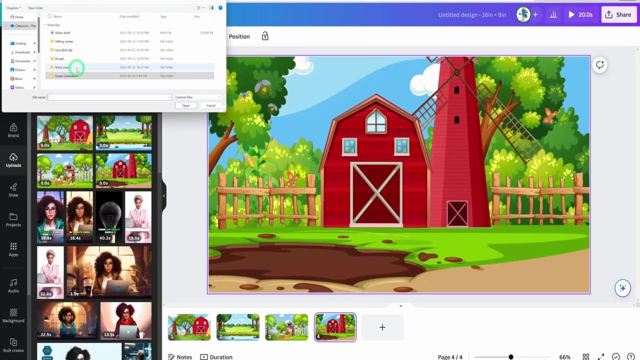 created according to each scene, and you might ask why? because we want to make sure that we sync it with the scenes and we also want to bring in the different animals according to when the voice is saying it. the next thing you need to do is go to upload upload files and then choose all the 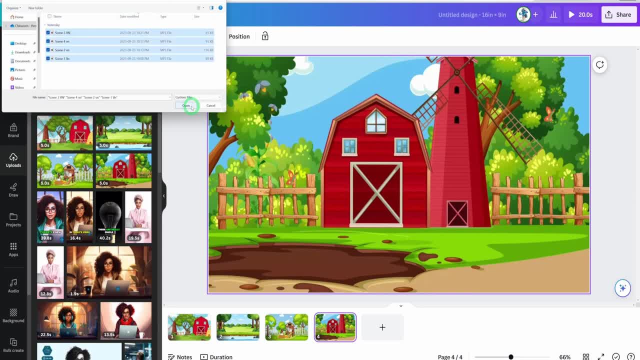 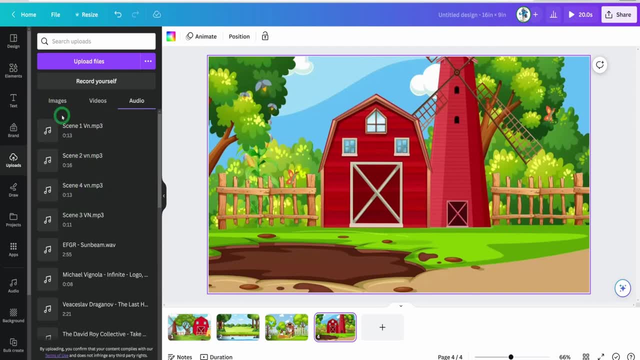 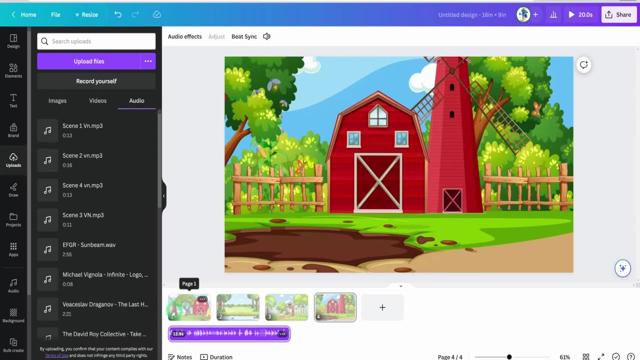 voiceover that you have done. i have four of them here so you could select them and click on open. i have them uploaded already. you could see here scene one, scene two, three and four. for the first scene i'm just going to drag the audio underneath it, as you could see here that it's longer than 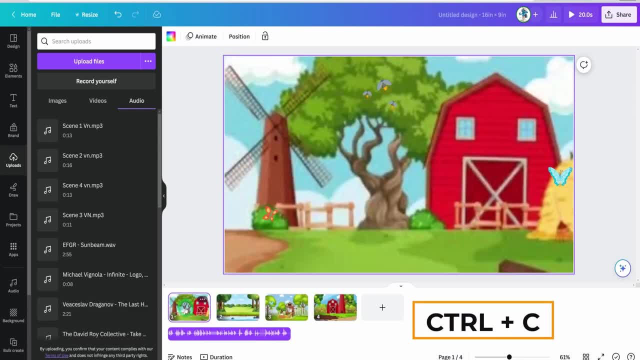 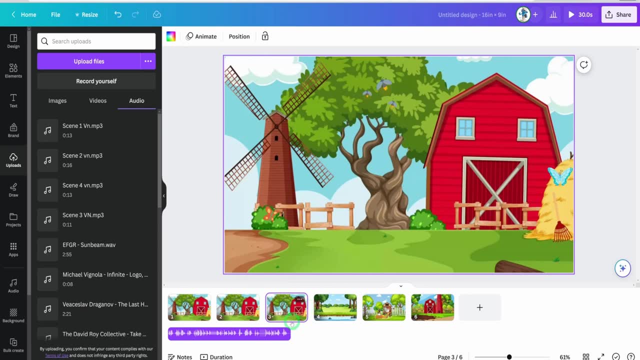 the first scene. what you could always do is click on ctrl c, ctrl v. it's going to paste. we do the same thing. you can see here that the volume of voice we have is also different, but as you can see here, it is a little bit smaller compared to the first two scenes. so we will just make sure that. 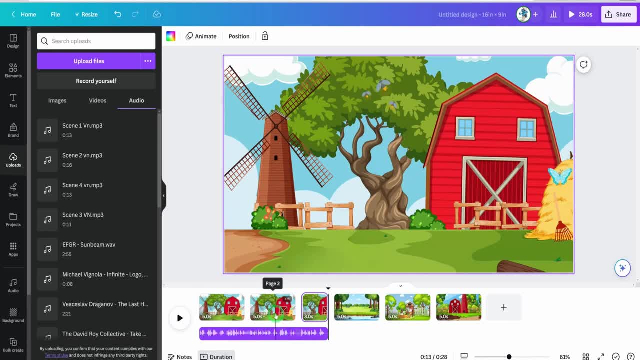 we match it with the size of the voice, so we'll just come here and reduce this a little bit to match the size of the voice. as you can see, all this matches the voice here. the next thing we're going to do is that, because here this is just the beginning scene, where we're talking about welcome. 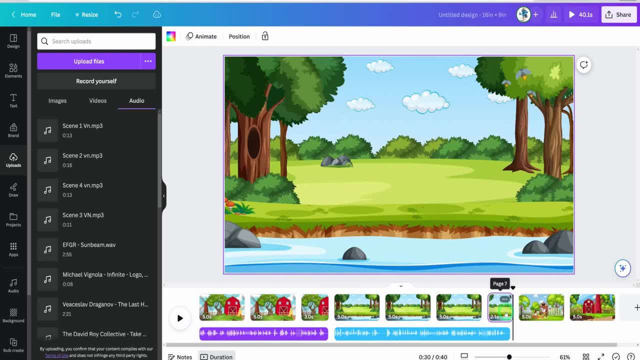 scene and then we make sure that we reduce the scene to fit where the voice stops. okay, the next thing here would be: because here we're talking about the cows and we have to put in the cows to animate it. you come to the beginning of the scene and we're going to look for a cow. you can. 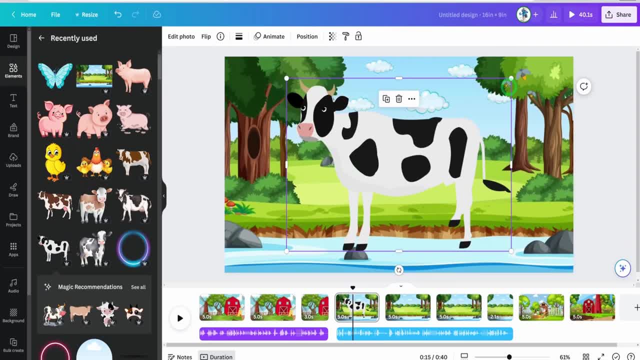 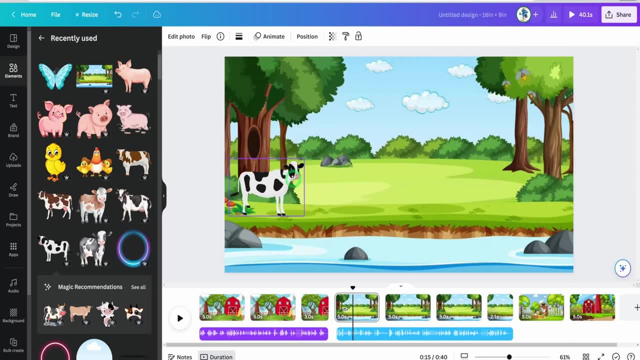 go to elements be using this. we just place the cow here and reduce the size, make it sit here and click on flip. let's flip it to face this way. take it all the way to the end. the next thing is: we want to animate this cow coming in while the voice is mentioning the cow. the next thing we 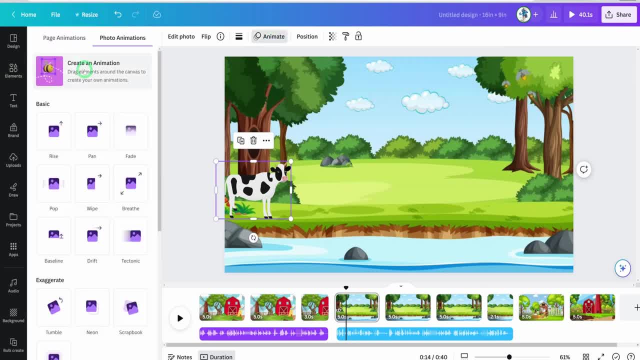 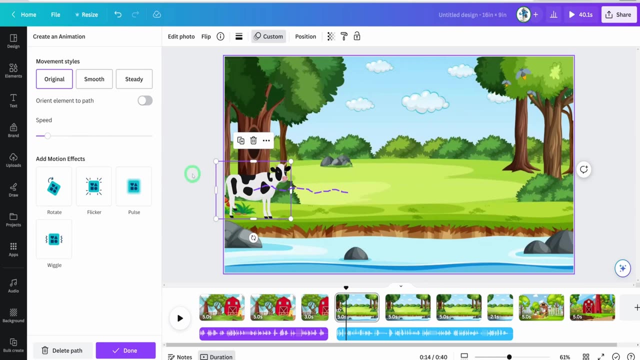 will do is we will click on the cow, click on animate and click on create an animation. then you're going to click on the image, hold and drag it to create a path, depending on what you want. just click on this and move it. stop here, okay, this. 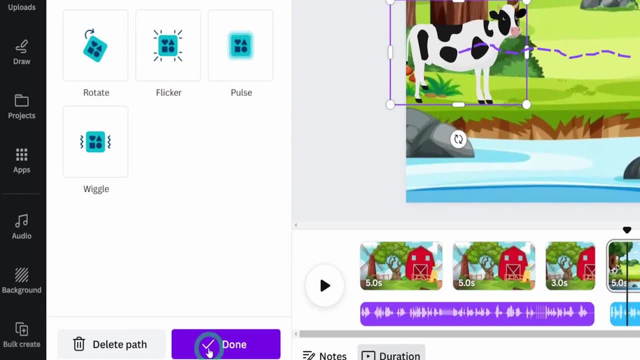 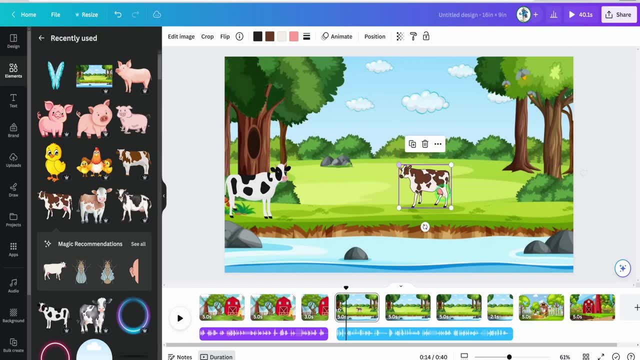 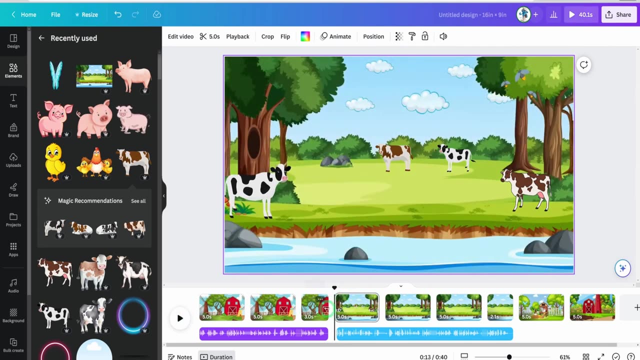 this, this, this, the next thing. we'll just click on done, since we have this, and then we'll go ahead and add a bit of other cows within the scene as well, just to give it a bit of context. okay, this is going to come in while it's playing. right, this is what you're going to do to repeat on all the scenes for the 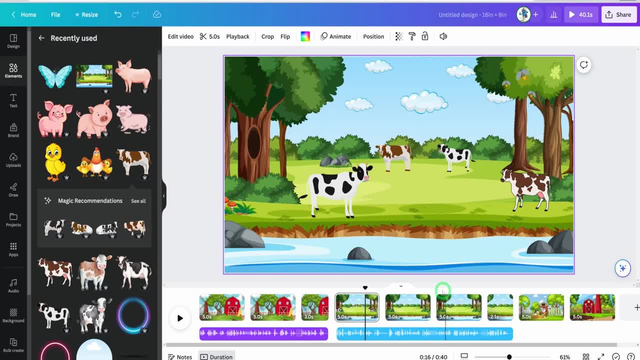 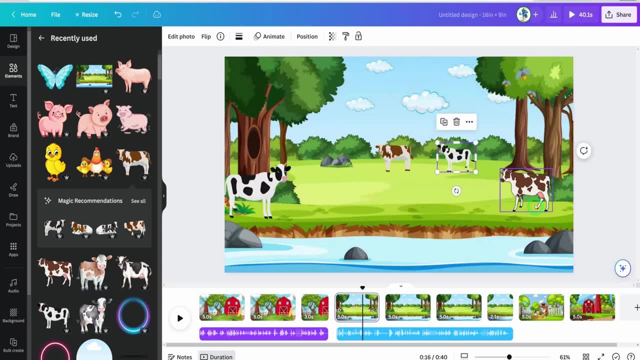 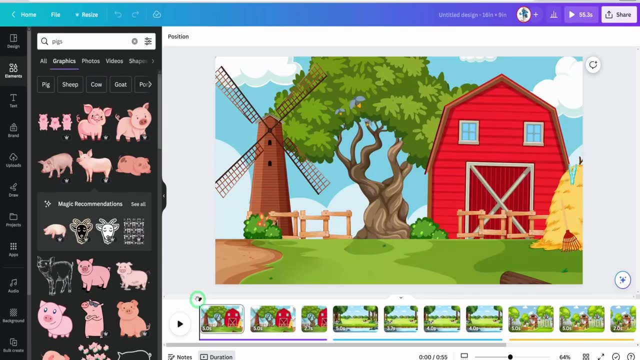 differences of when the voice is mentioning which farm animal that it's showcasing. as you can see that here this scene is blank. what you could do is basically just copy the cows that you have here and paste in those scenes. give it the same aesthetics. i've gone ahead to put in all the scenes. this is the. 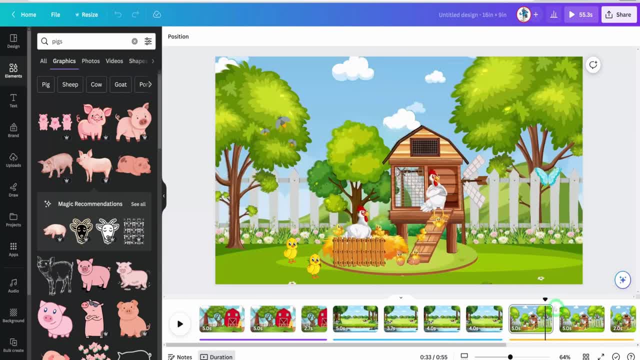 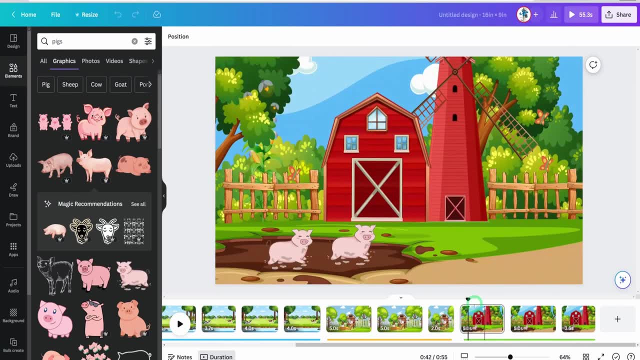 cow we talked about. this is the chickens- the same animation process that i showed earlier- and then this is the pigs that i used with the animation and the movement as well. once this is ready, then we are done with canva. the next thing we need to do is to create a new animation. 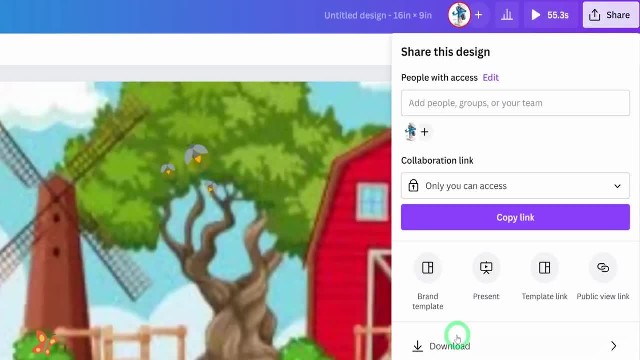 so create a new animation and click on this video. i will be using adobe express animation preview. the next thing we're going to do is to download this as an mp4. you go to share, go to download and we'll download it as a single video. make sure that this is up to 4k quality and select. 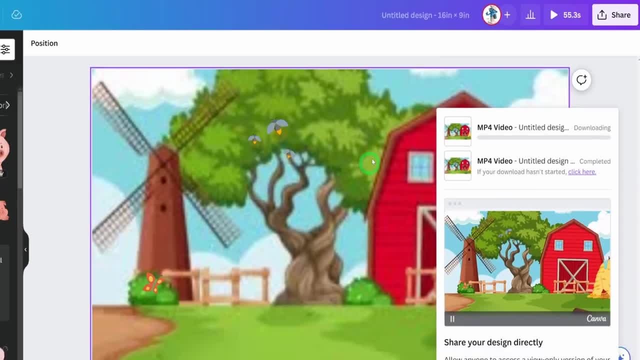 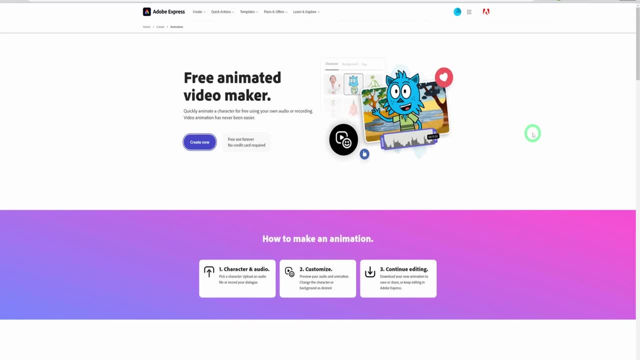 all pages and hit download and it's going to download this to your computer. while this is downloading, the next thing will be for us to generate our talking ai avatar. so create our talking ai avatar. we'll be using adobe express animation. it's currently free. it has characters. 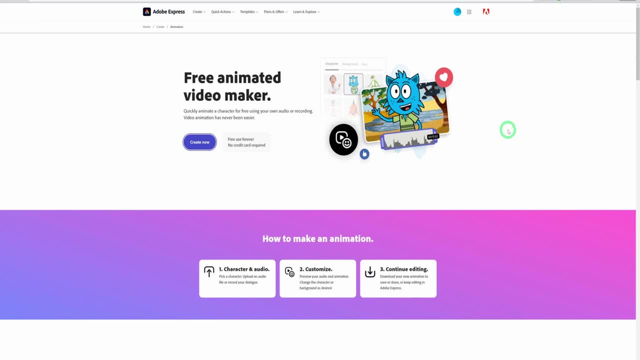 that are good for children's educational channels. once you've downloaded it, we're going to click on the children's educational channels and you'll see that you can create a child's adult channel as you to sign in. it's for free. just click on create now and it's going to create and open up to this page. 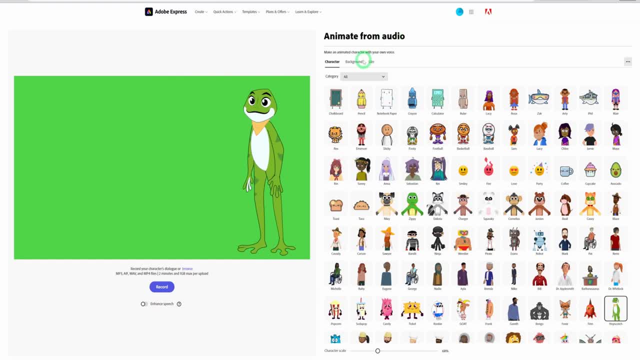 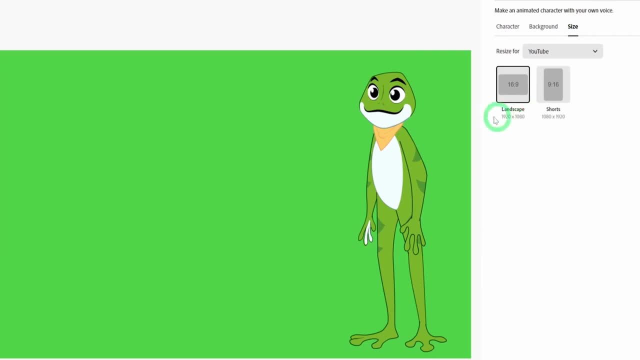 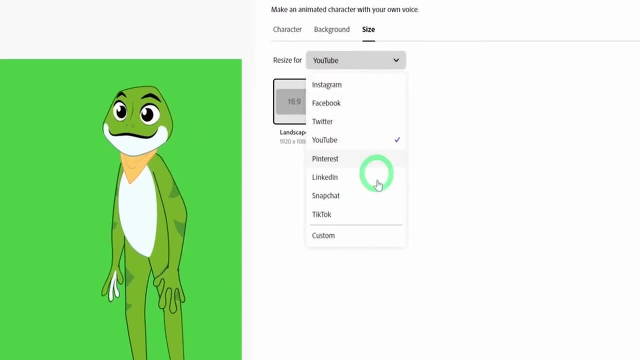 because i have already set this up and let me just show you what i did. you could choose a particular character. this is the character i chose- hopscotch- and then for the size, i chose a landscape size because it's for a youtube video and we wanted to have the same size here. you could choose different. 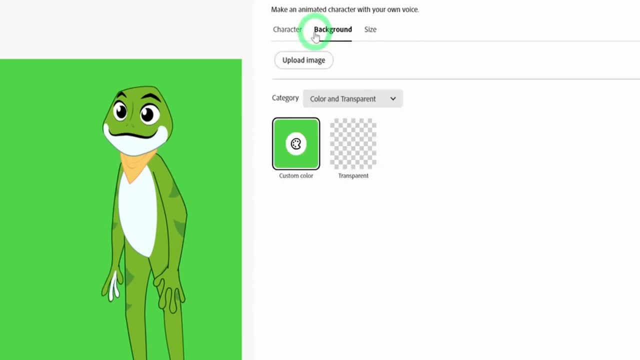 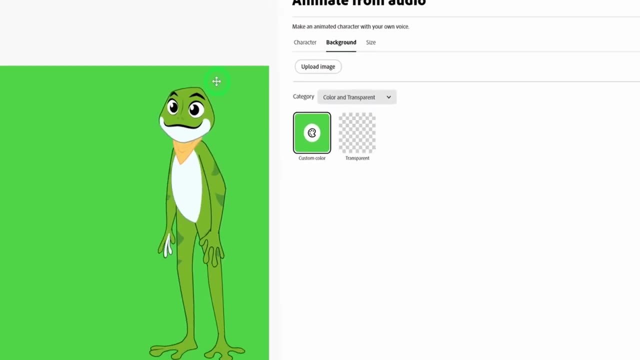 sizes of different videos you are trying to create, and for the background, i chose it to be green because we'll be using this in our editing tool and i will show you later how to do that. this is the character we'll be using. i placed it here because, as you could see from our scenes, the 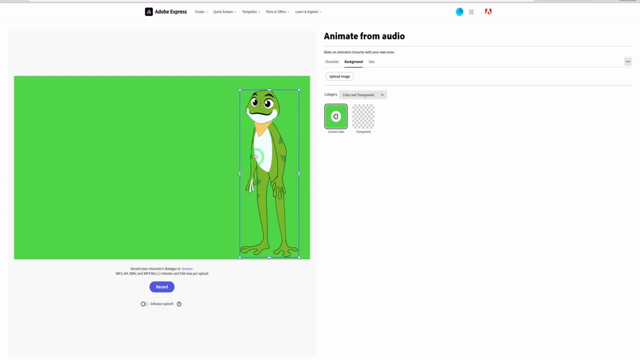 animals are coming in from the left and the talking avatar would be on the right. the next thing to do is to click here that says browse, because we want to animate this avatar. so we'll click on browse and we'll be choosing voice over one and click on open. it will go ahead to upload this and try. 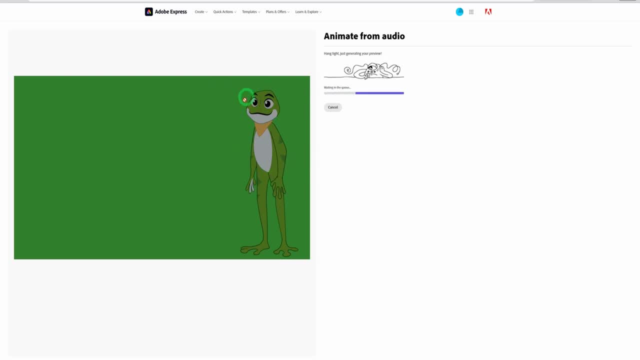 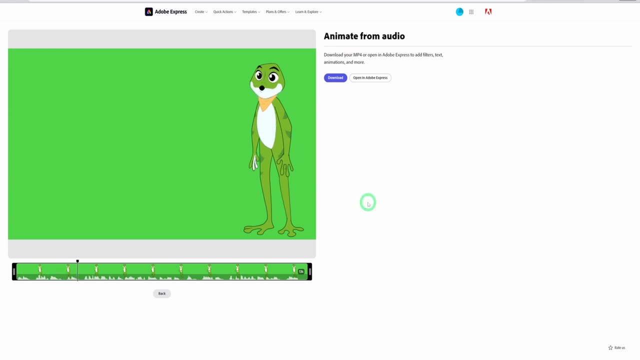 to lip sync what the voiceover is saying with our animation. just wait for this to finish up. so this is done and let's see how it sounds. hey there, little explorers. today we're visiting a very special place where we meet some of the friendliest faces on the planet. yes, we're at a farm. let's discover who these friendly. 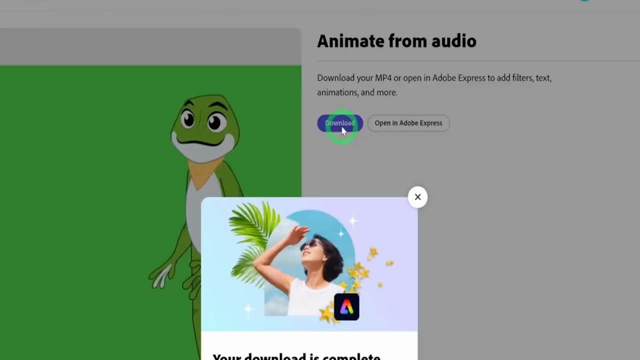 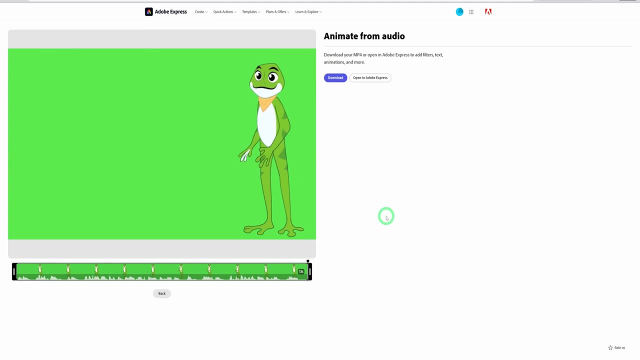 faces are, shall we? okay, just click on download and it's going to download to your computer. you go ahead and do this for all the scenes that you have, one after the other, and download them to your computer. the next step is to go to your computer and click on download, and it's going to download. 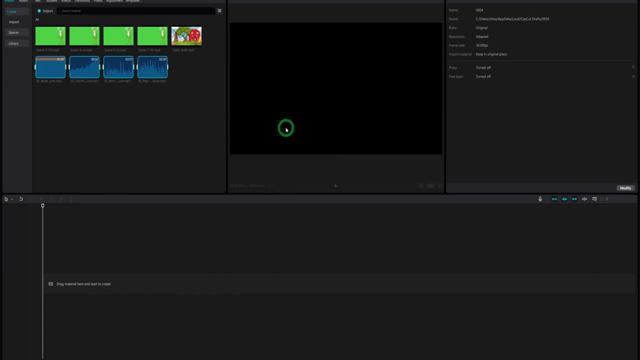 this part. so here is where the next step is to edit all that we have generated as far as we're coming to capcot, open and create a new project and drag in all the videos and clips that we have generated. this is the video drafts that we have. you just drag it to the timeline. these are the characters. 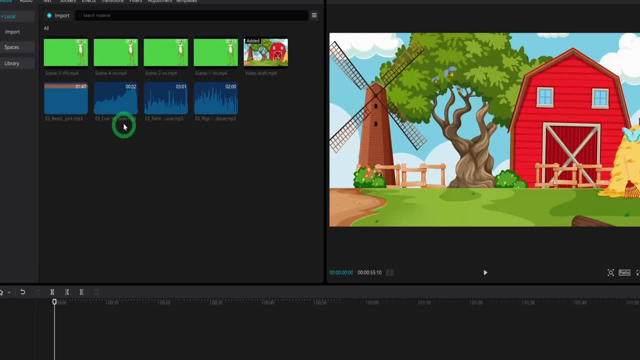 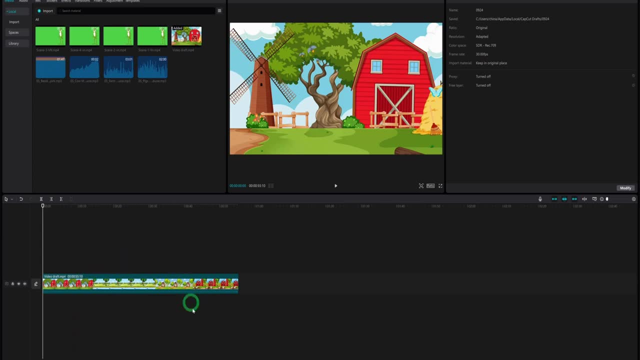 that we generated. that is here, and this is some of the music and some sound effects that i want to use to tie this all together. now that we have dragged this into the timeline, we'll just go ahead and cut through into four scenes that we have generated and then we'll start placing 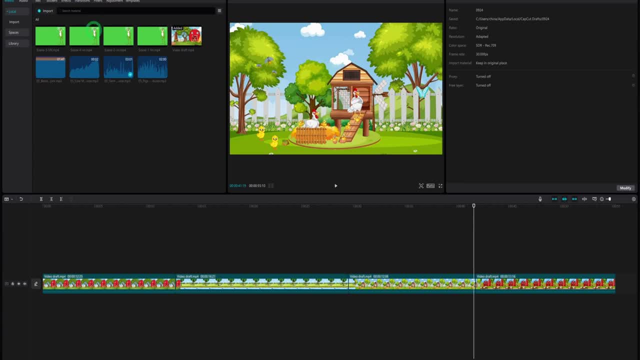 these talking avatars over the scenes. next thing is to place these talking avatars according to different scenes. as you can see, they are named accordingly. just drag this over the first scene. make sure that this aligns. once we come to the first scene, you would notice that the green screen 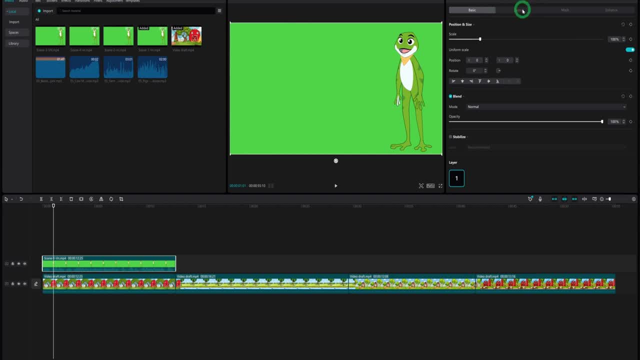 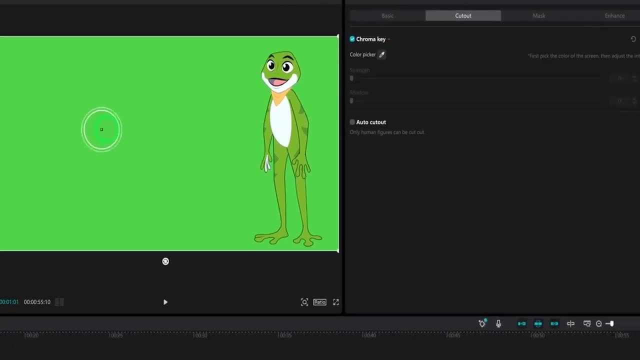 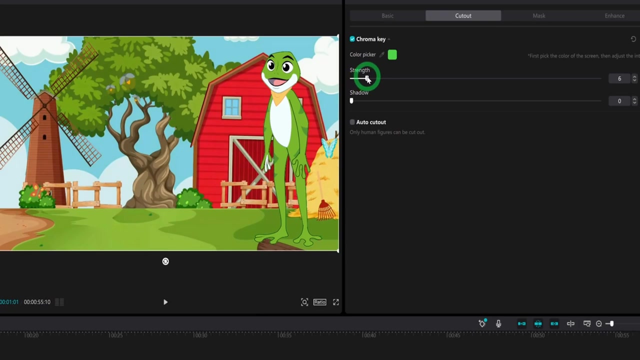 is overshadowing the images below it. what we're going to do is: you come here that says cut out, click on it. click on chroma key and use the color picker. pick the green and then the strength. just reduce the strength and, as you can see, the background shows, just reduce a little bit. 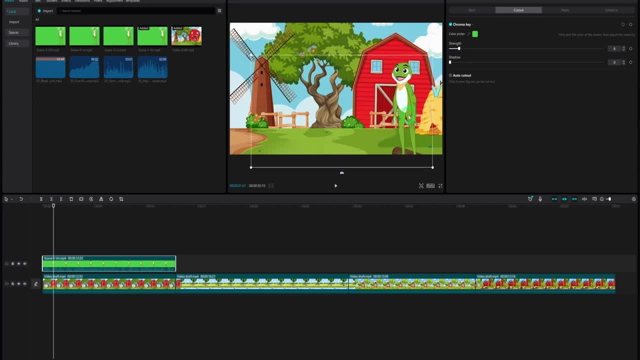 and then here we're going to reduce this little guy. just place it in such a way that it's okay, increase this a little bit. this looks really nice. you go ahead and do the same for each scene. okay, we are done placing the talking avatar over the screens. just go ahead and just put in the 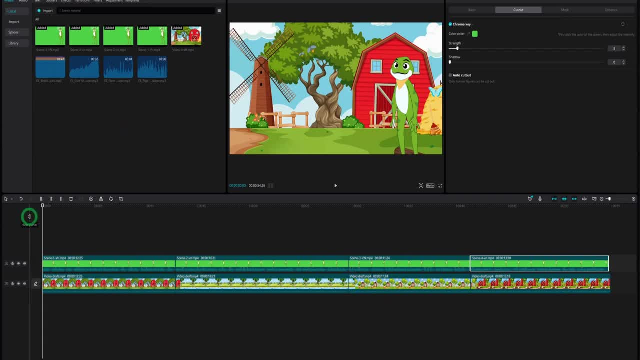 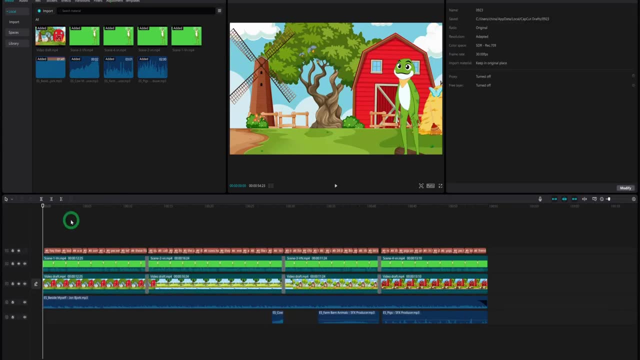 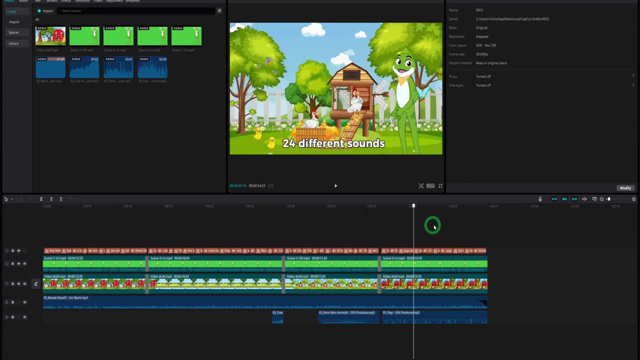 music, some sound effects and some transitions. we'll go ahead and put in the subtitle and we're good to go. i'm gonna head to put in every single thing you could see. it has its own subtitle. the sounds, the transitions, everything is there. the next thing you need to do is to click on export and choose. 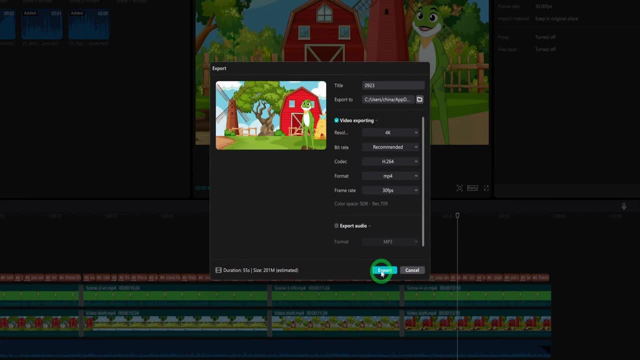 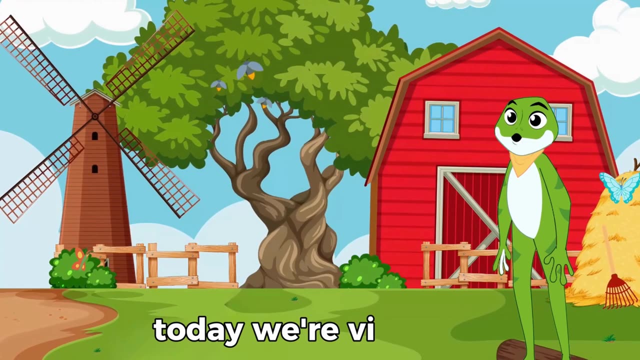 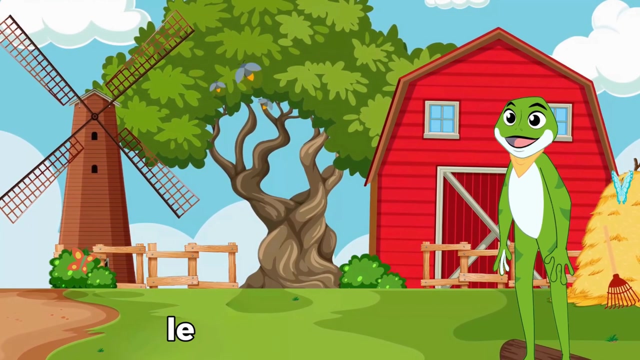 the format that you want it to be hit. export and the video will be exported to your system. this is the final result. hey there, little explorers. today we're visiting a very special place where we meet some of the friendliest faces on the planet. yes, we're at a farm. let's discover who these friendly faces are. 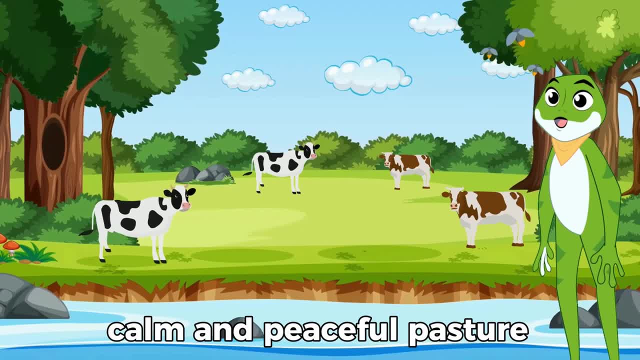 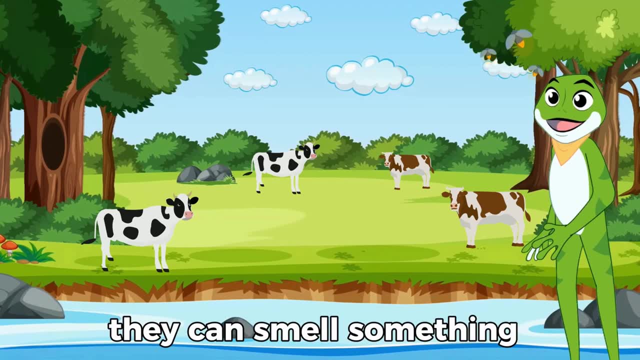 shall we? our first stop is the calm and peaceful pasture where our big friendly giants, the cows, are. did you know that cows have a fantastic sense of smell? they can smell something even from six miles away and their milk gives us yummy things like cheese and ice cream. let's say moo to thank. 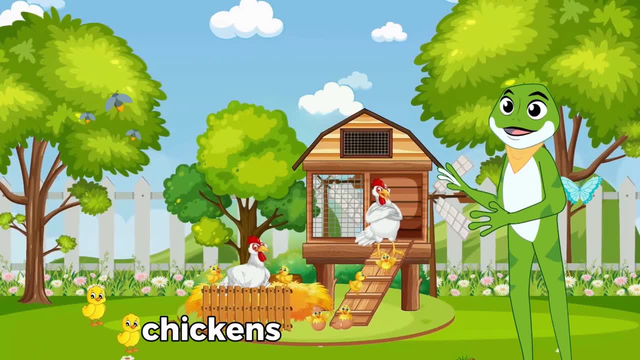 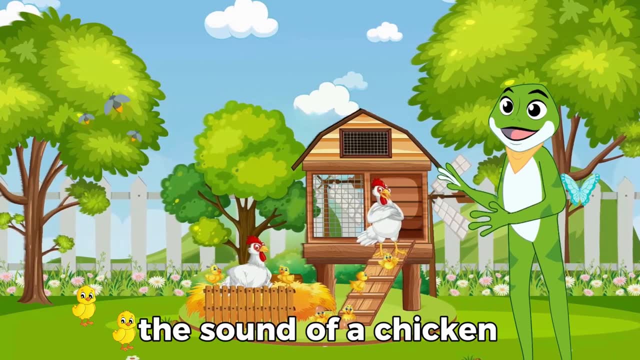 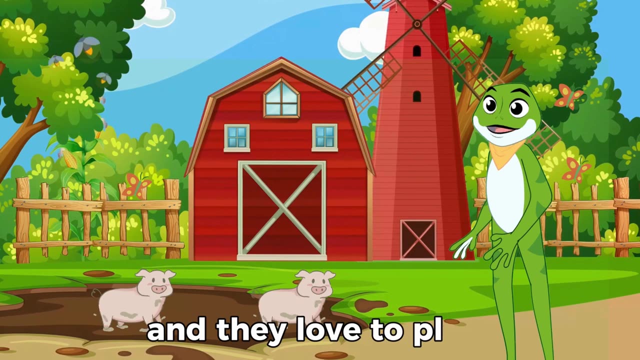 our cow friends. next up is the lively chicken coop. chickens are amazing. they communicate with each other using over 24 different sounds: bach, bach, bach. can you make the sound of a chicken? let's try it together. now we're visiting the super smart pigs. pigs are very clean animals and they love to play in the 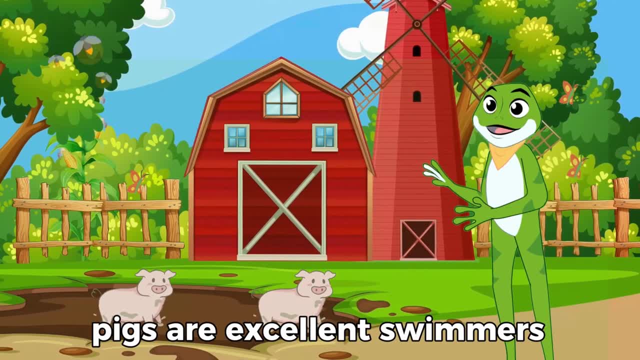 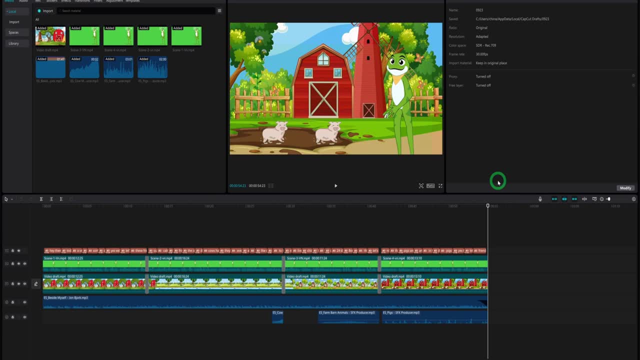 mud to keep cool. did you know that pigs are excellent swimmers? yes, they are. let's give our pig friends a big oink oink. hello, looks really good. next thing you need to do is just to create your youtube account and upload your video to your youtube account and you can see that the 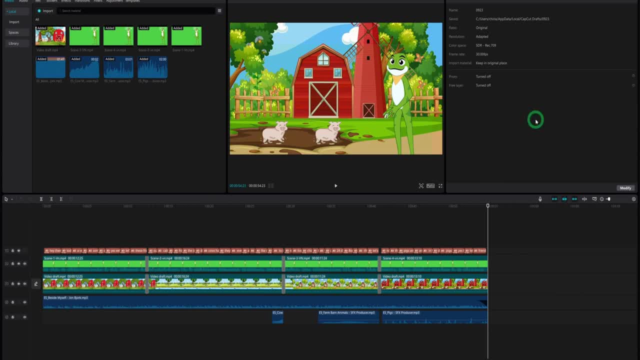 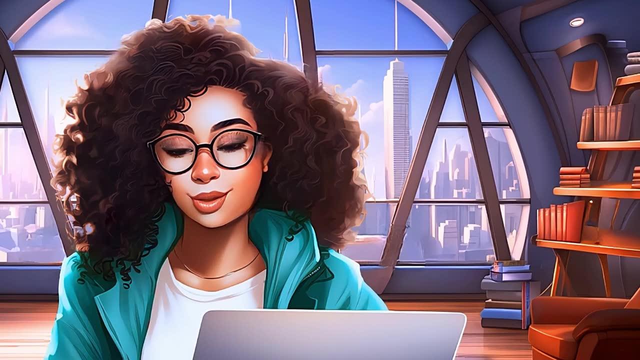 videos and you could repeat the same process. remember, consistency is the key. if you're interested in creating more fun and interesting animated story videos, check out the video at the top right and for other businesses that you could actually start with the help of ai, you could check. 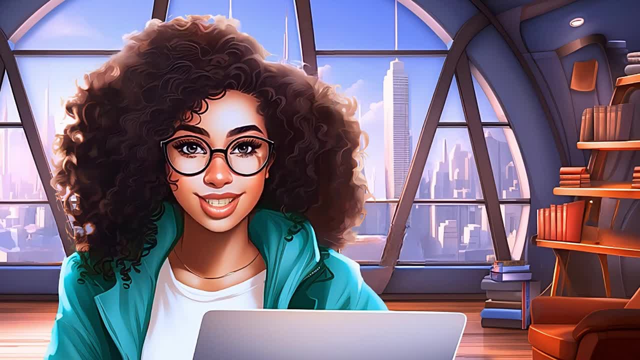 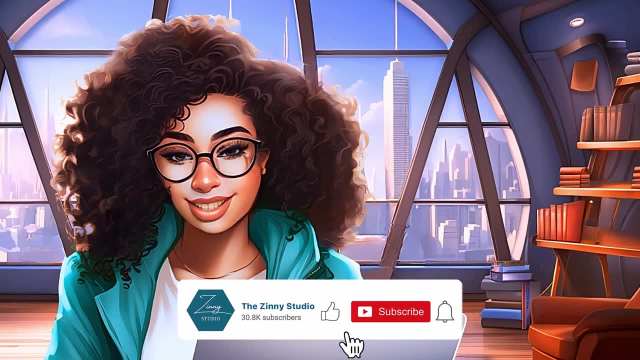 out the video in the bottom right and in the next video we'll be continuing that series on a couple of products you could sell within this q4 to help you make some passive income. and do not forget to like and subscribe and turn on your bell notification to know.